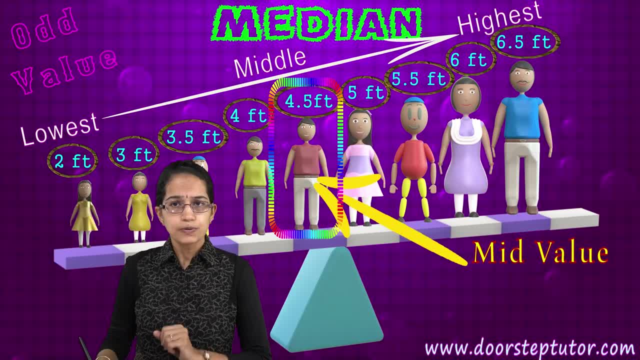 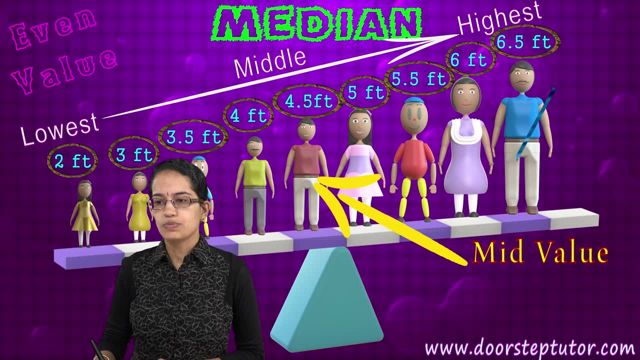 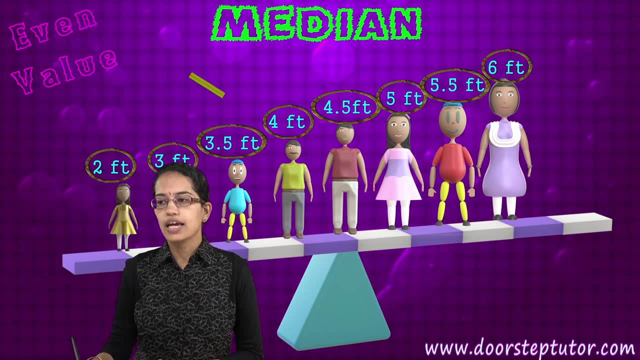 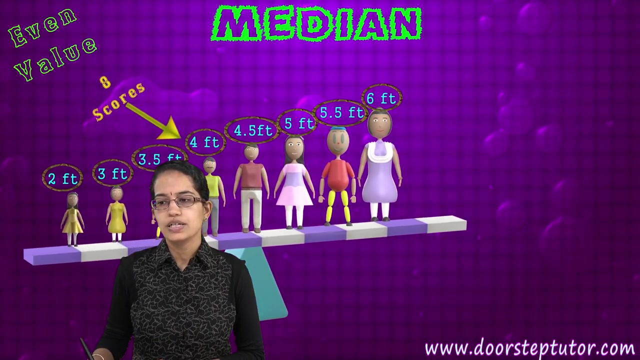 That's there, And the 5th value is the mid value. However, what would happen when the scores are even numbered? So let's say I remove 6.5 and I have even scores there. So I have these scores which are here. Now, these 8 scores that are there, What would be the median for this case, For the even values? what I do is n by 2th score and n plus 1 by 2th score. 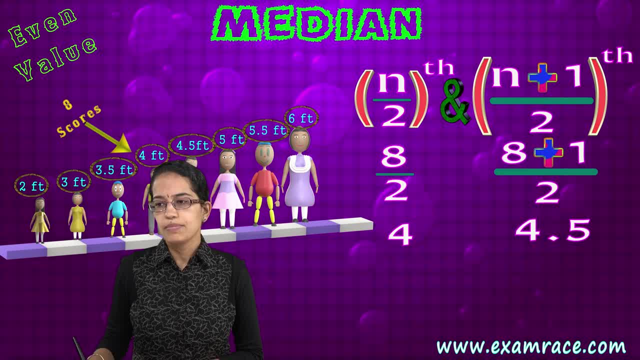 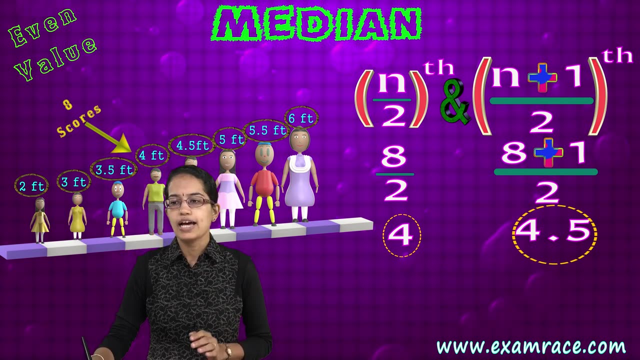 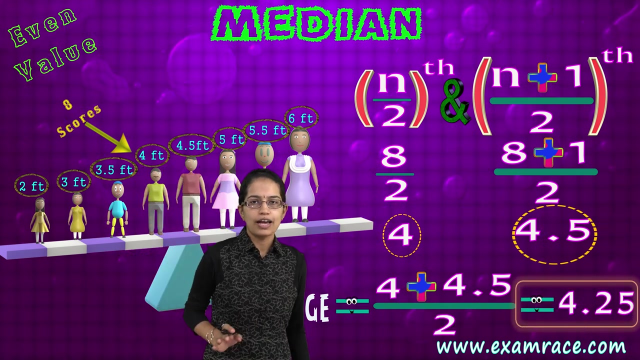 I take the average of these 2 scores, So what is the n by 2th plus 1 score? So it is the 4th value and the 5th value. I leave 3 values from each of the side, So I have the 4th and the 5th value. I take the average of the 4th and the 5th value, So I take the average of 4 plus 4.5 divided by 2.. So it's 4.25. And this 4.25 is my median, which is the middle value of my score. 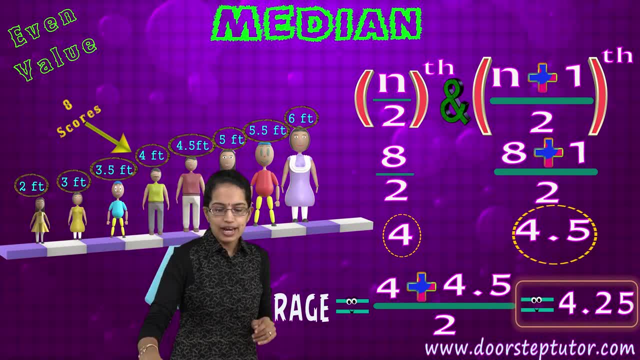 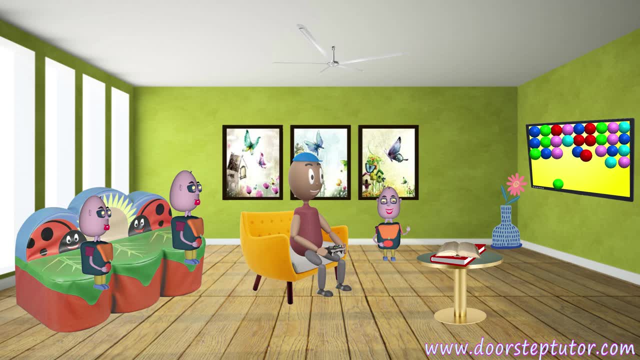 Now what would happen? let's say I take another example. Now. this example is pretty interesting. I have a child playing a video game. Now in the video game he has to shoot on to the range. When he presses the buzzer there is a shoot. that is done, So he presses the buzzer on the following seconds. let's say 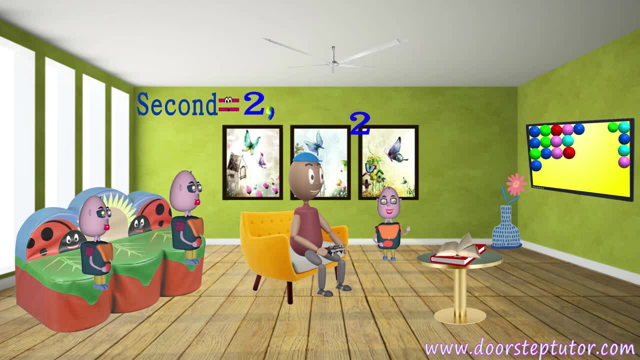 So the presses are at 2 second, 2 second, 2 second, 3.5 second, 4 second, 5 second, 6 second, 7 second, 8 second, 9 second, etc. second, and one of the presses takes, let's say, 10 second because suddenly there was a call from the. 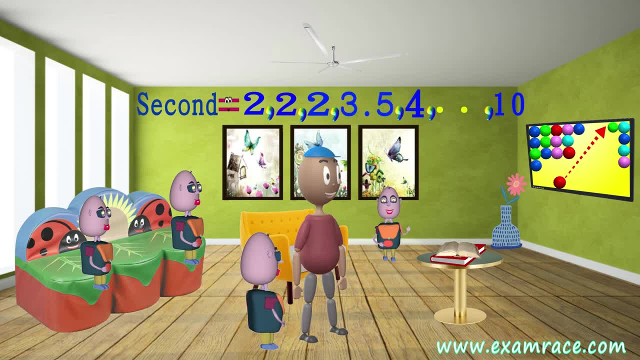 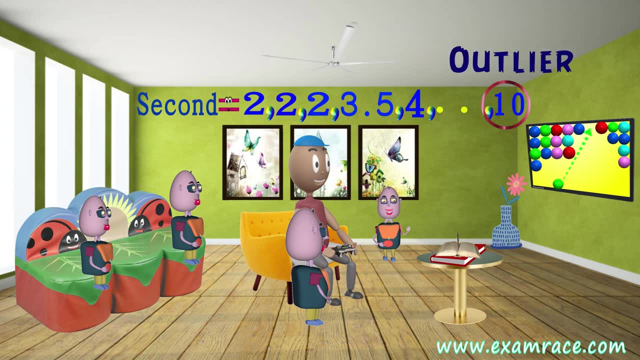 mother, or there was another friend who came in and disturbed him. so in this case, what happens is this value of 10 becomes an outlier value. it is a value that was because of the distraction that was caused while playing a video game. now this outlier, when it comes to mean what i would do. 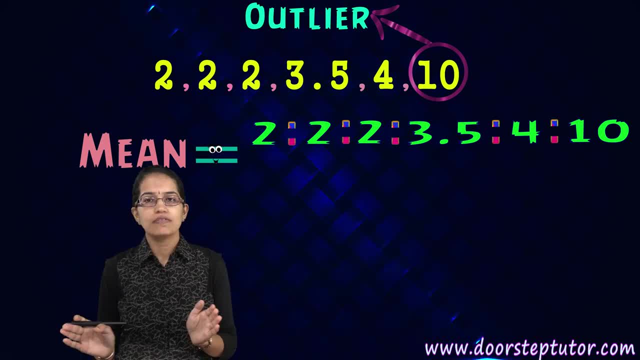 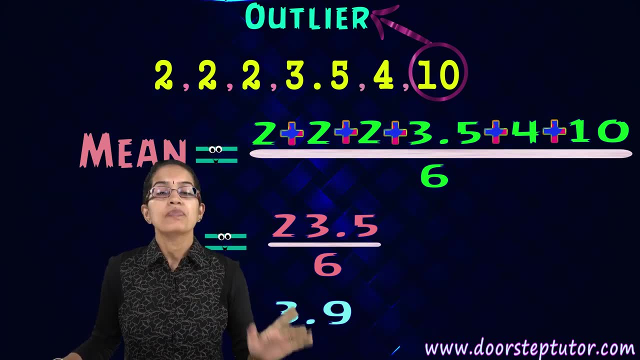 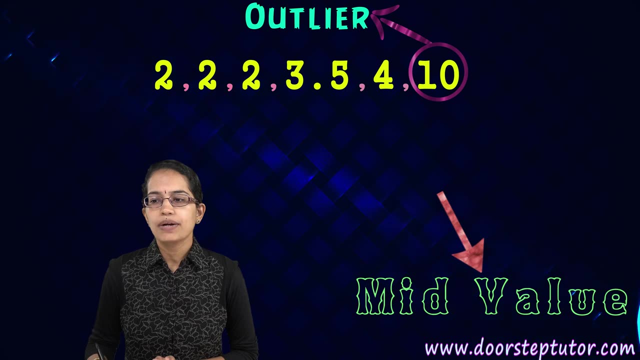 i would take all these values. i would add up all the values and divide it by the total number of values, so this outlier value would be counted in the process of mean. however, when i take the median, what would happen? i have to simply find out the mid value. so the mid value would be the average of 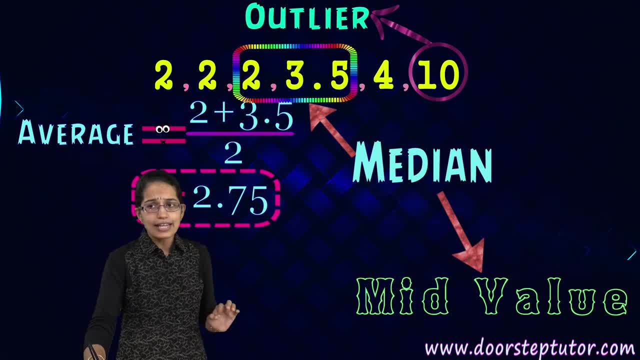 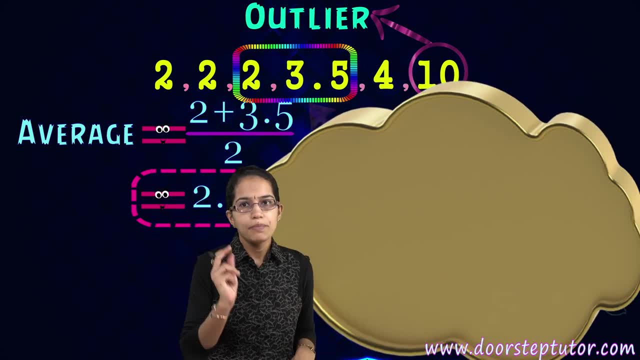 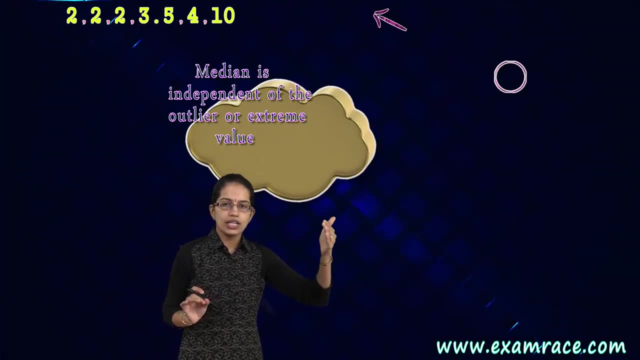 2 and 3.5 in this case, and that would be my median, which is my average value. so, in very simple terms, i would take all these values, i would add up all the values and divide it by the total number of values. median is independent of the outlier or the extreme values. let's talk about the last example. 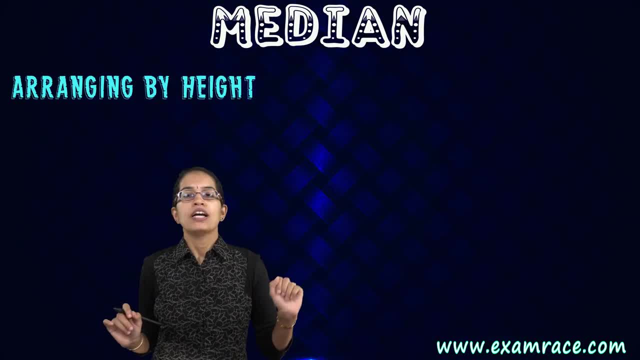 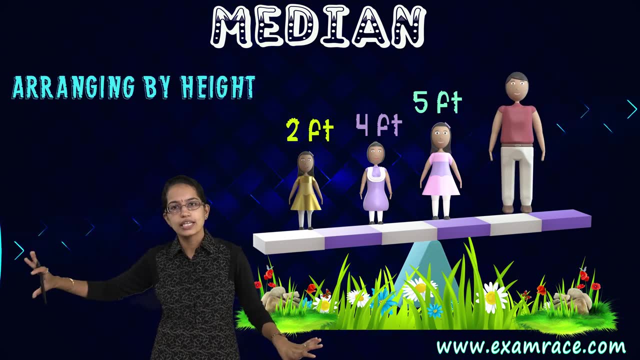 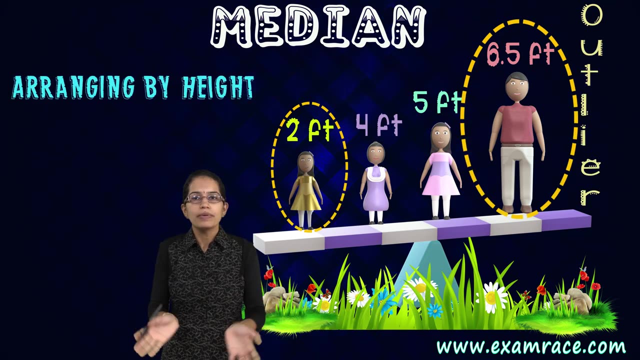 that we did, which was arranging the kids by their height. so definitely a kid of two feet in height, adult of two feet in height and a person of, let's say, 6.5 feet in height are outliers, are extremes. you won't find it a normal circumstances, so those extreme values are ignored. 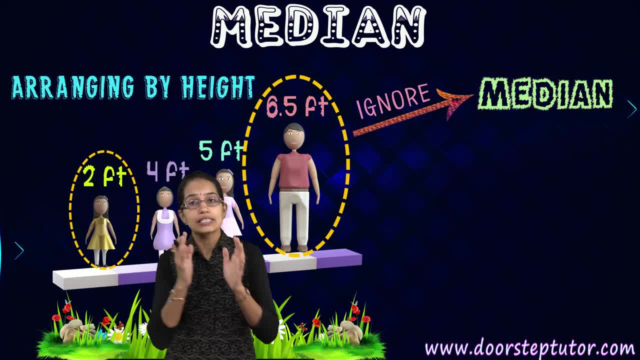 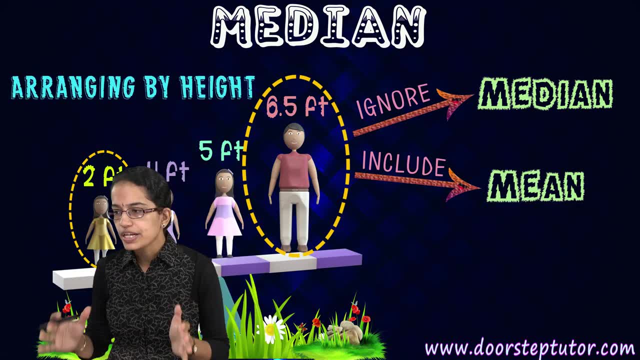 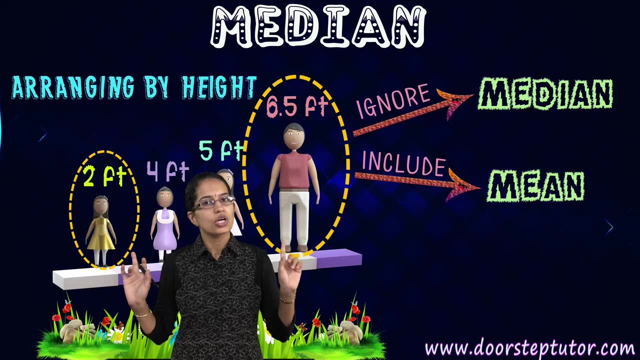 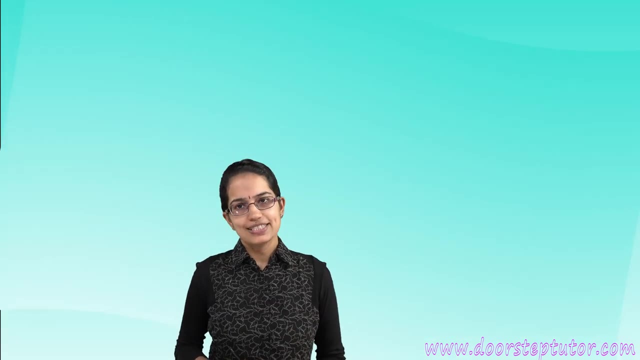 in the case of a median, but those extreme values are part of your mean or the average that you calculate. so it's very, very important to understand that median de-emphasizes any kind of extreme values or outliers that are there. now let's talk about another measure of center tendency and this: 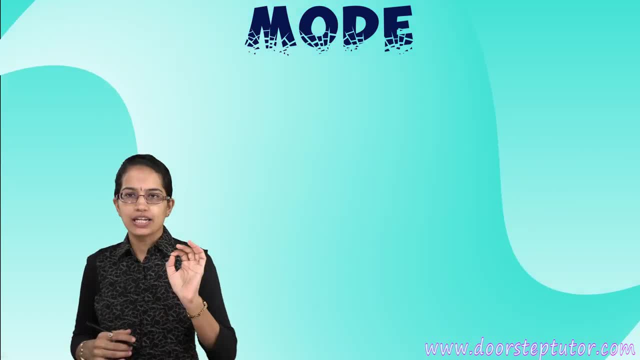 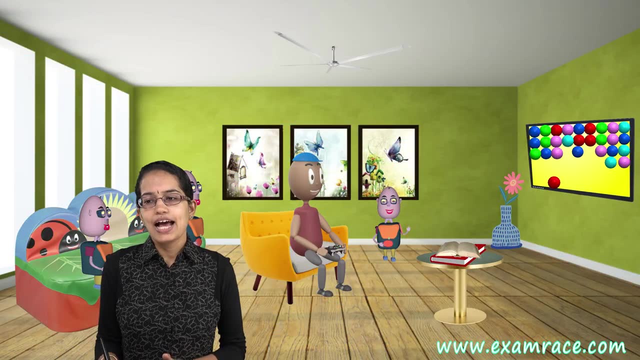 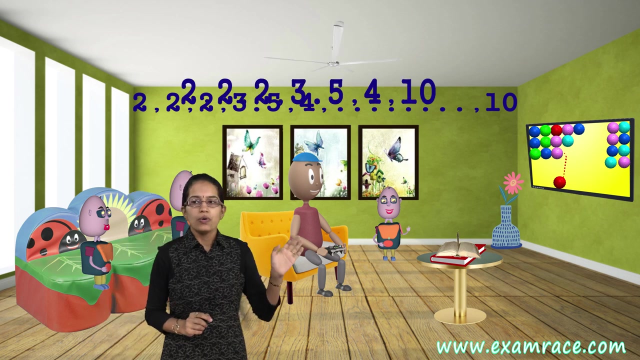 is mode. mode is a very, very important characteristic. with the same example of the video game, let's say: the child has a reaction time where he is able to press the buzzer at the following seconds. now, in the same example, what is the mode? mode is 2 in this case, because it is the 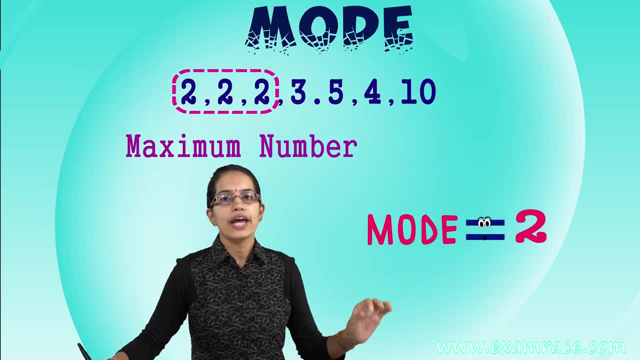 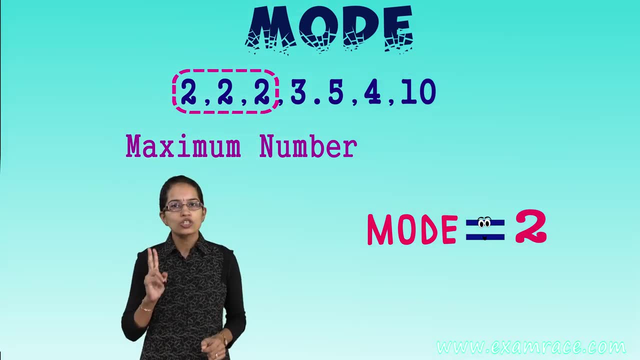 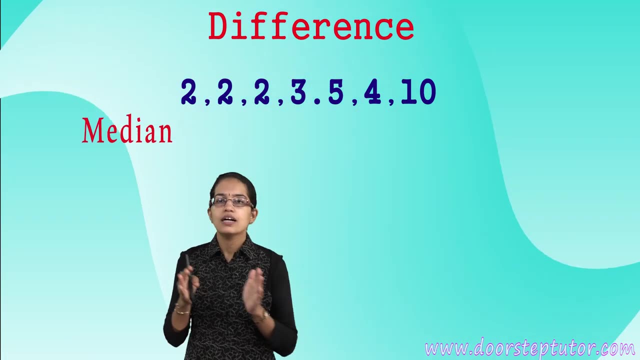 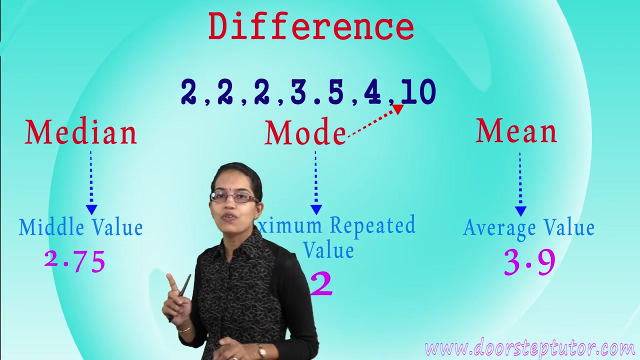 maximum number of instances that the boy has. so most of the time he is able to press the buzzer at 2 seconds and therefore this 2 second becomes the mode. so very, very clear. what is the difference between a median a mode and a mean mode? again, is independent of any kind of outlier values. 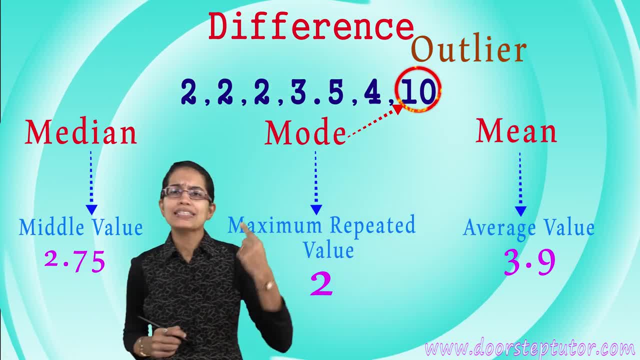 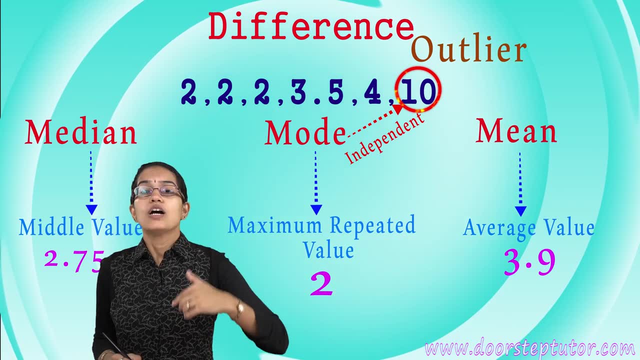 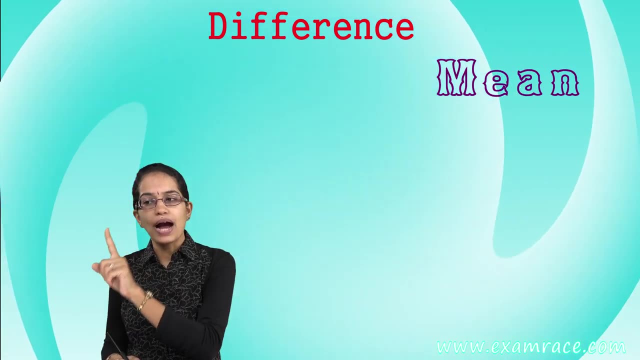 that are there. in this case, 10 is an outlier value, but since it's only once, it's independent of that outlier value. however, what would happen in the case of mean, with the same example as explained before? the mean would be affected by any of the extreme. 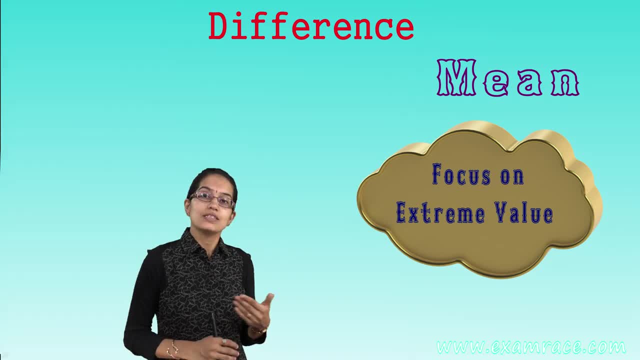 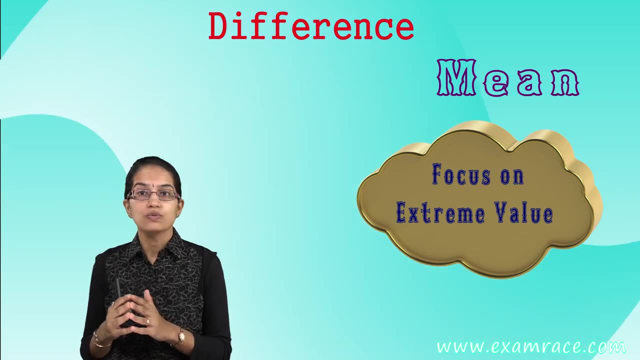 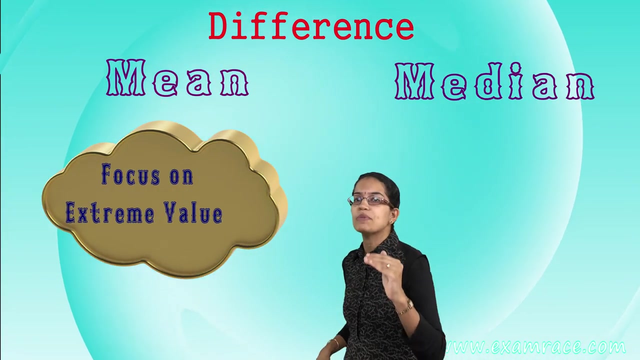 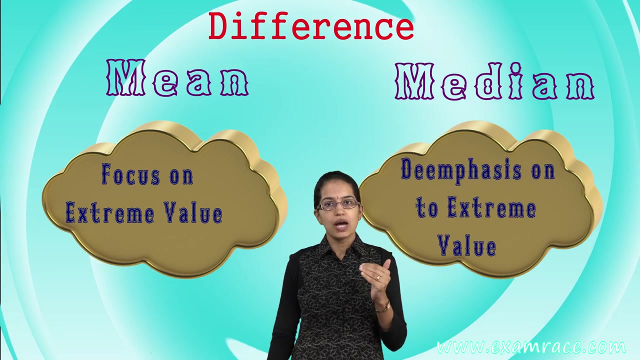 values and therefore sometimes it is believed that mean is a measure of central tendency which is commonly used, but the most common thing that we understand is median is considered as a much better representation because it has an idea to de-emphasize on to the extreme values. 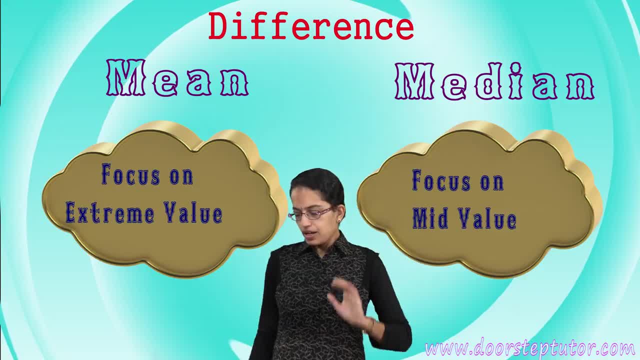 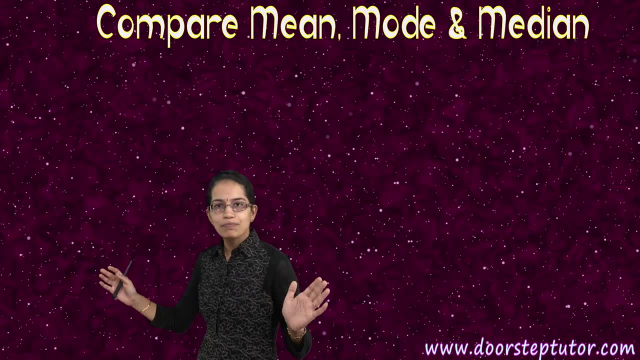 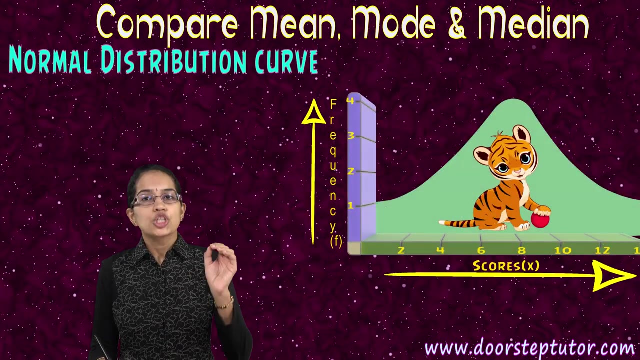 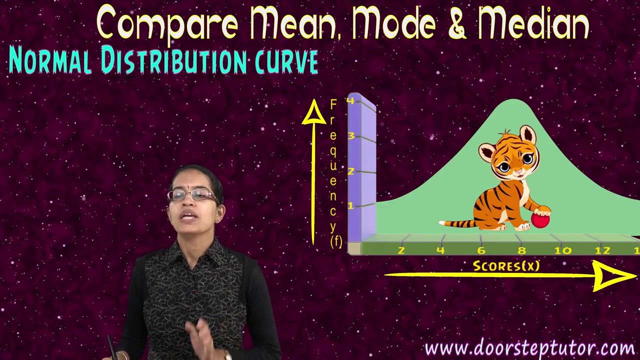 and focus on to the mid value that is there. the next thing is the most interesting aspect: comparing the mean mode and median. we have already talked about the normal distribution curve, the concept of skewness in cretosis, in our previous lectures on the introduction to statistics, so you can just refer that back. in a normal distribution curve, what happens is the mode. 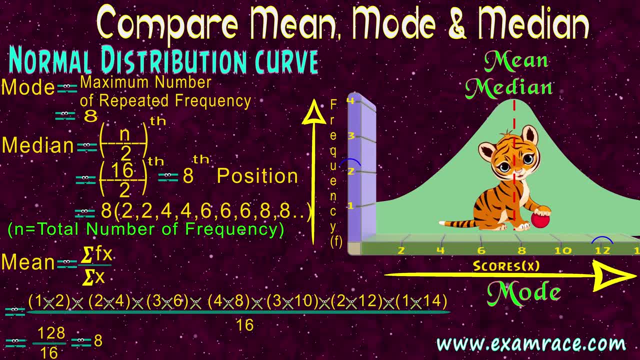 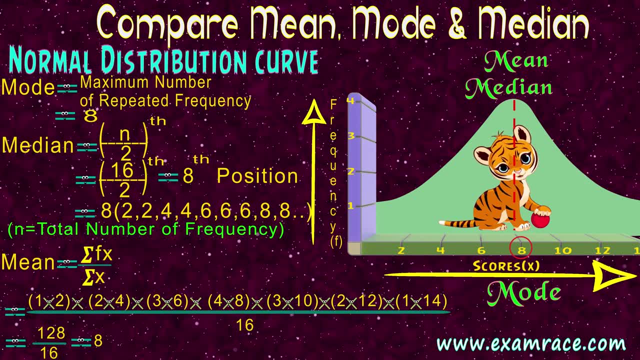 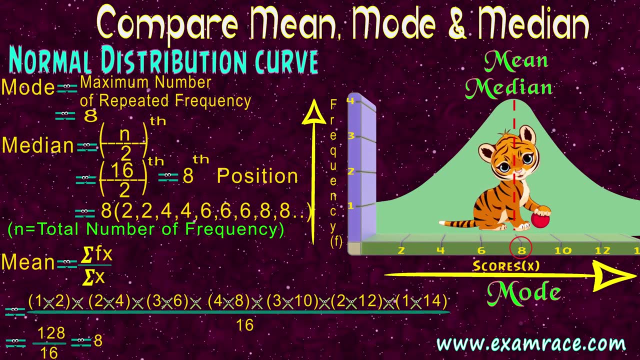 of the median and mean. all of them are at a common location. why, in this case, when it is a normal distribution curve, my mean value would be the middle value, because it can exactly overlap, as we have seen previously. so this is the mean value. again, this is the place where you have highest number of frequencies. 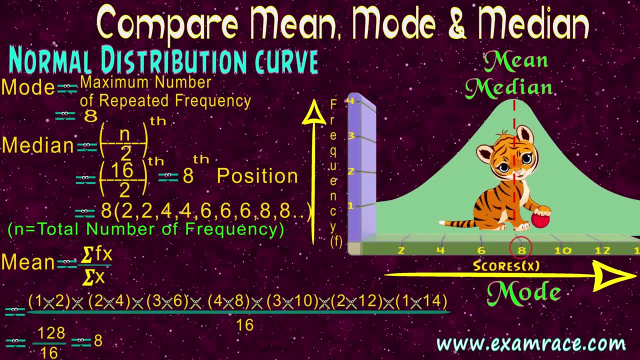 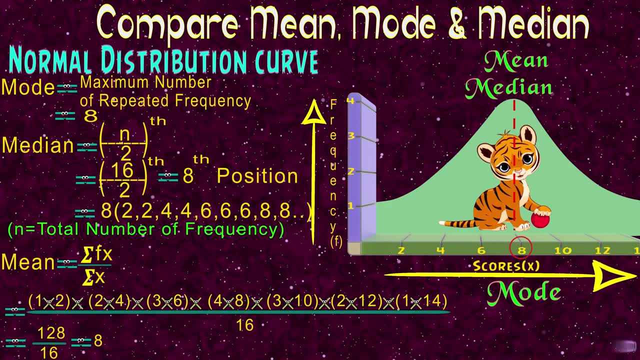 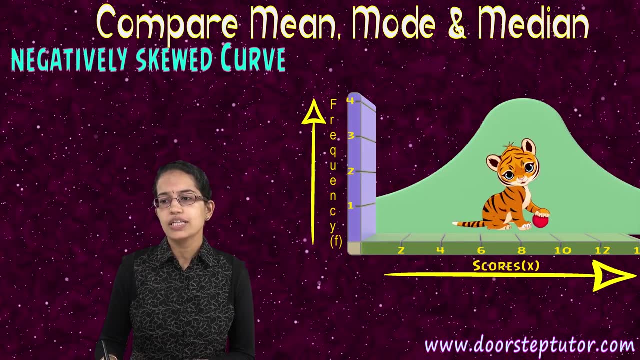 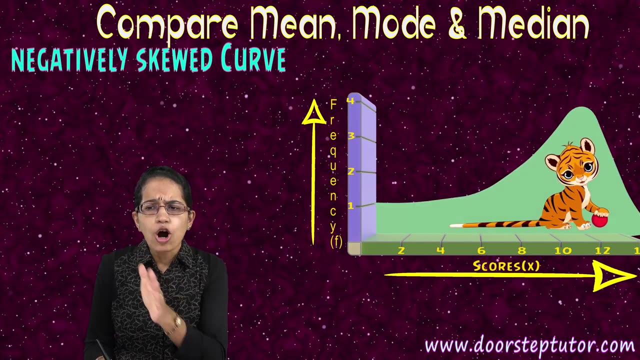 so mode is again here and obviously the mid value is in the between. so you have the median also same position. so the mean mode and median are equal in this case. Next comes the example of negatively skewed. since it's a negatively skewed distribution, you have lots and lots of values which form the tail now, since there are lots and lots. 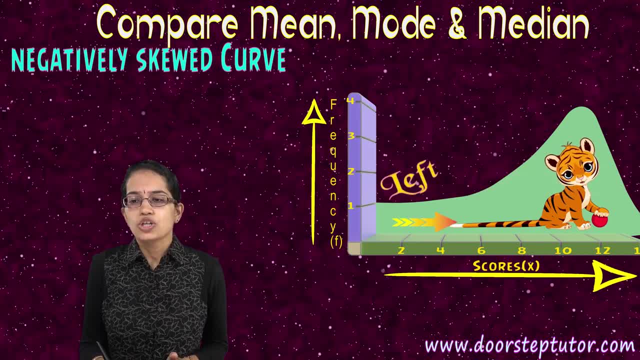 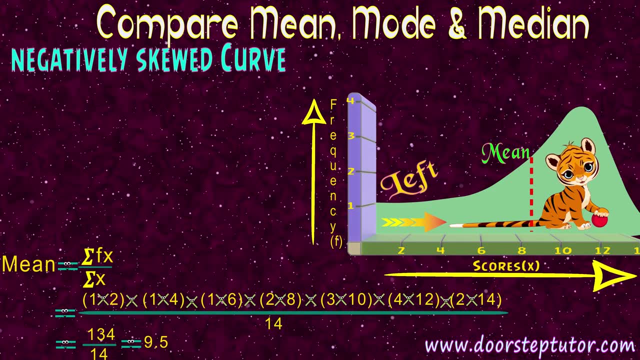 of values. on this side we call it as left skewed, so you have mean that would be closer to most of the values that are there, because you have a long tail and you have numerous values here, so the mean or the average would be closer to the tail. obviously. this is the 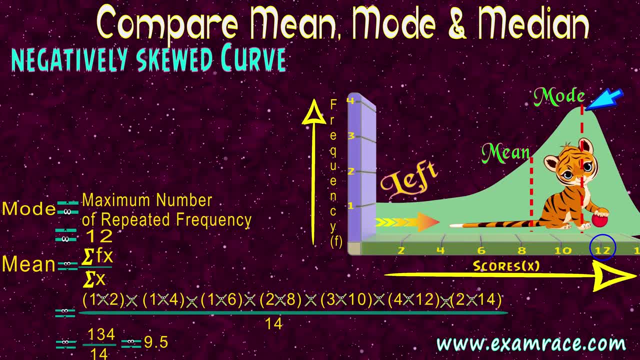 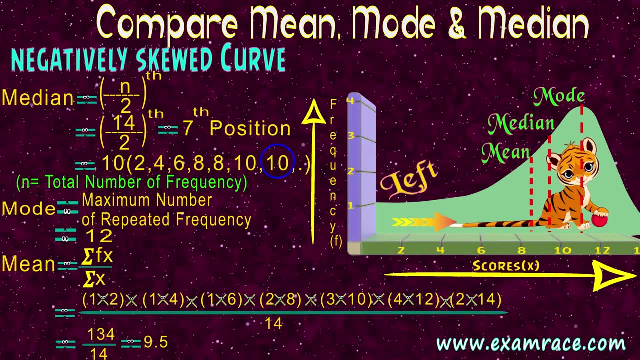 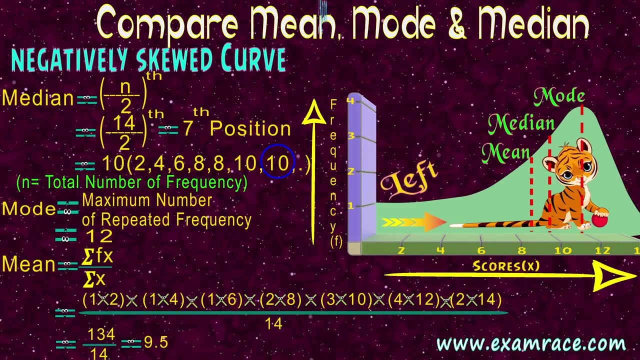 mode, which is the frequency, the highest number of instances that are recorded, and mid value is the middle value or median is the mid value that is there and that would fall exactly midway between the total number of instances taken. So in this case we say mean is less than median and this is an example of negatively skewed. 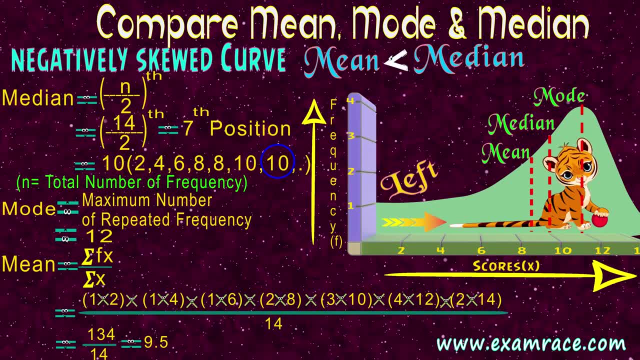 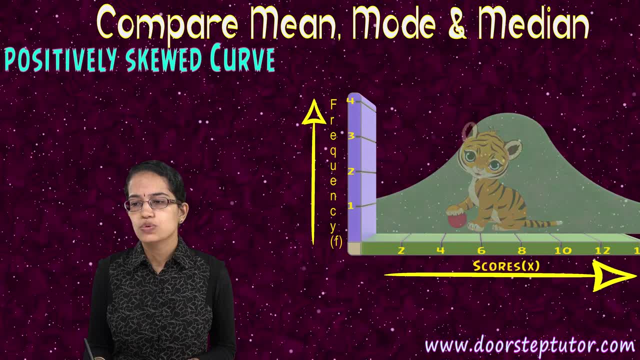 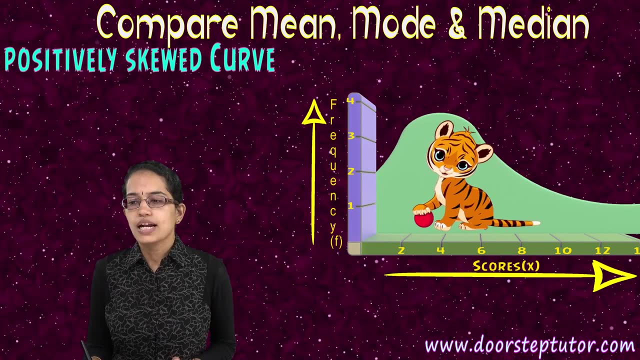 curve Clear. in this case there is no perfect overlap. that is seen as in the normal distribution curve. The next is a right or a positively skewed curve. so under a positively skewed curve you have numerous values that are towards the right, since there are numerous values towards. 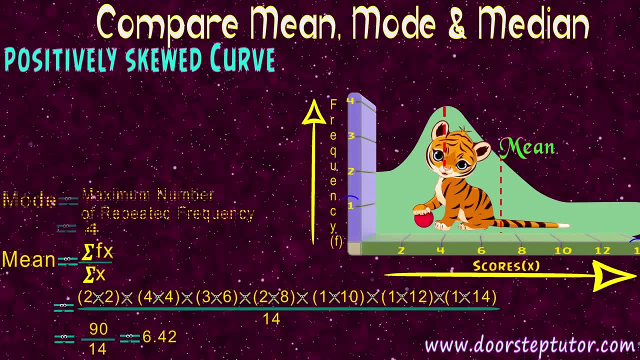 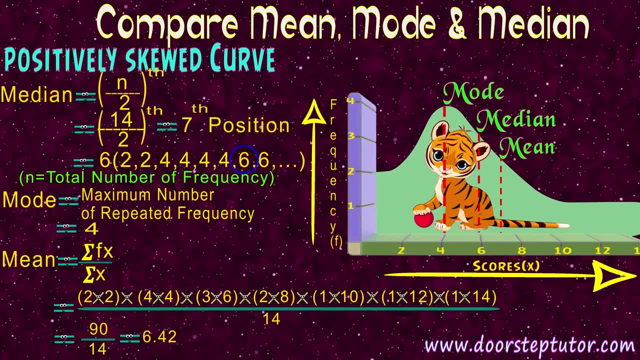 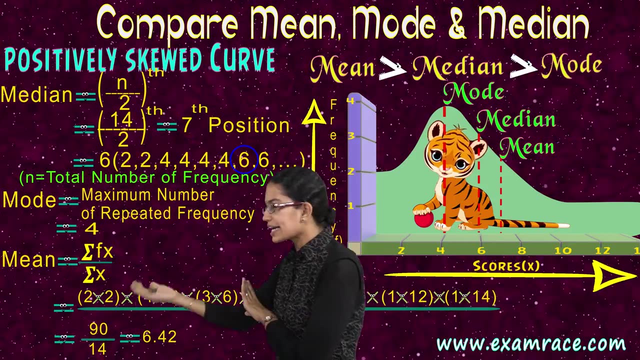 the right, your mean would be towards the right. your mode would definitely be here, which is the highest instances, and this would be the median. but in this case your mean value is much higher than the median value, which is higher than the mode. So the difference between a negatively skewed curve and a positively skewed curve is now. 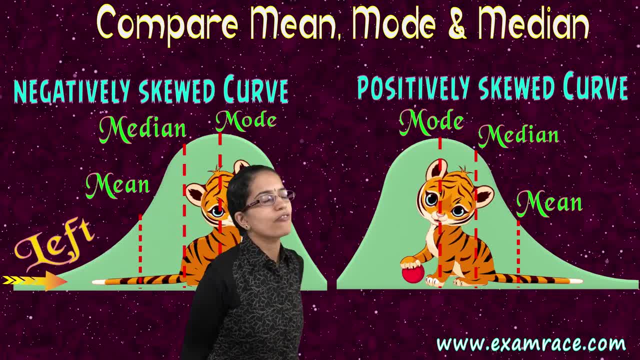 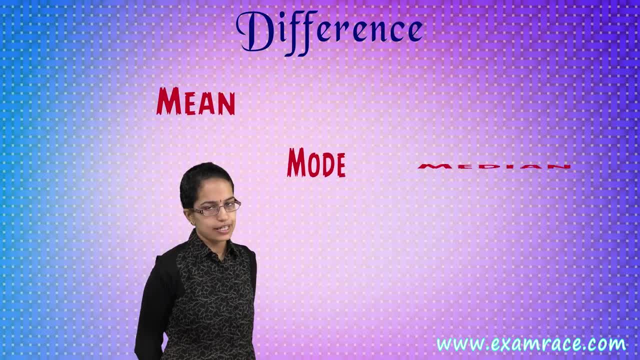 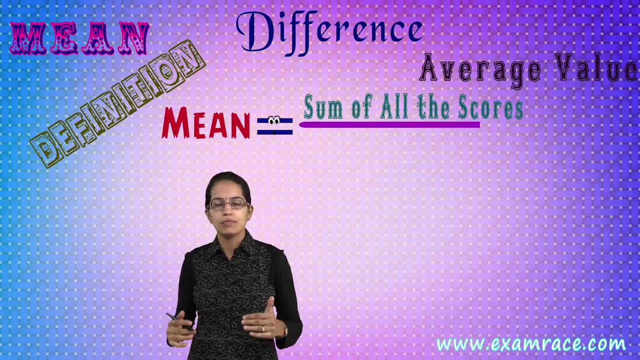 very, very obvious. The next important quick recap of understanding the measures of central tendency are understanding the difference between the mean mode and median. So mean, I repeat again, it's the average. so the sum of all the scores divided by the number of scores would lead to the average. 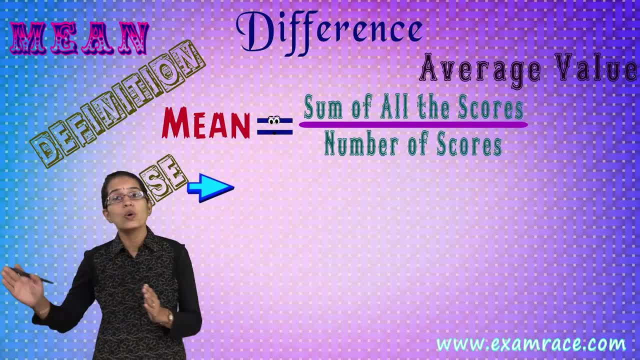 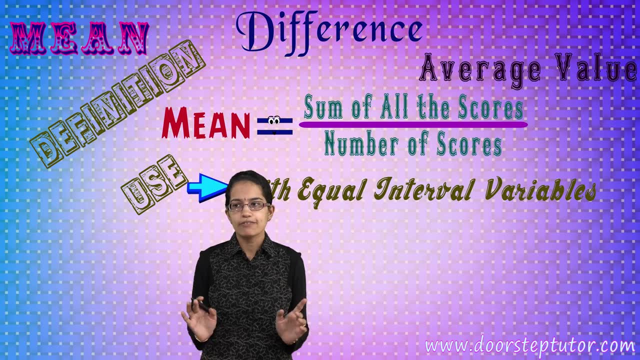 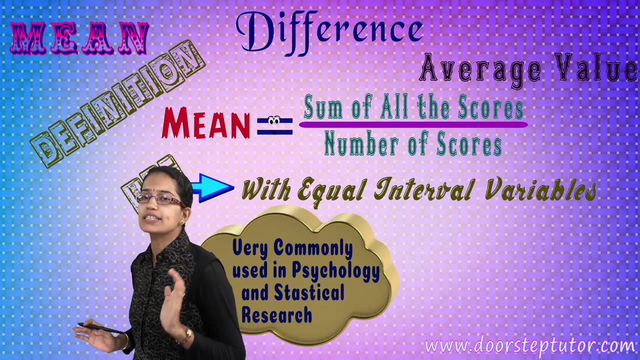 The average would be equal to mean. this mean usually has equal interval variables. so every 5th and 10th and the spacing that is there is equal interval and this mean is most commonly used in all psychological research or any kind of statistical research that are there. 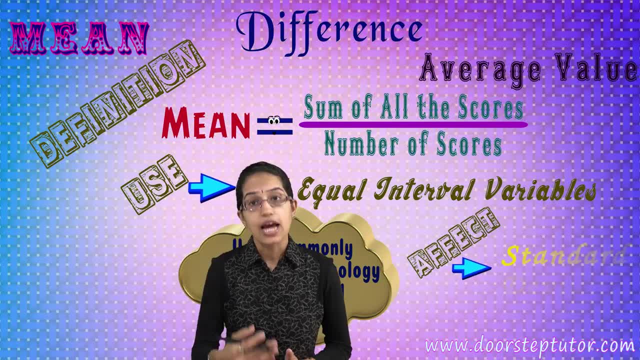 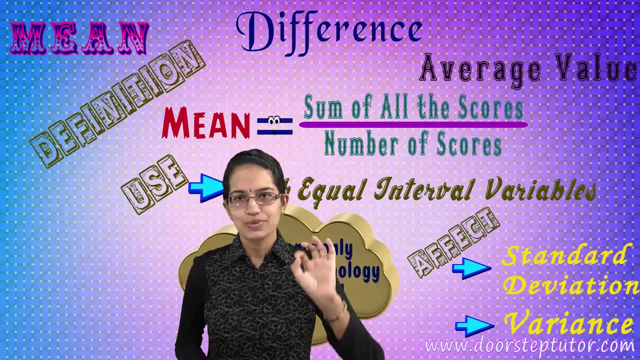 Now let's consider a fact where you have to calculate the standard deviation variance. all of those would require Mean. So Mean is the foundation stone. So this is the foundation stone, must and must know it. The next is mode. Mode means the greatest frequency, The highest. 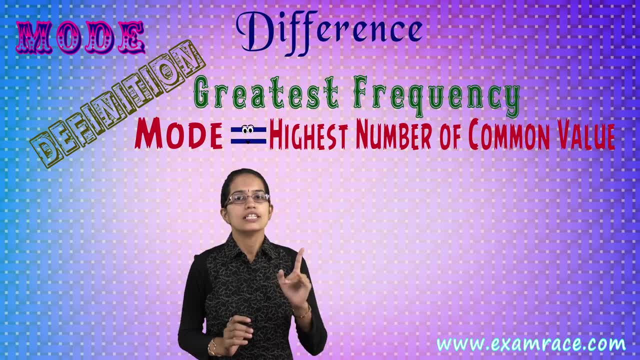 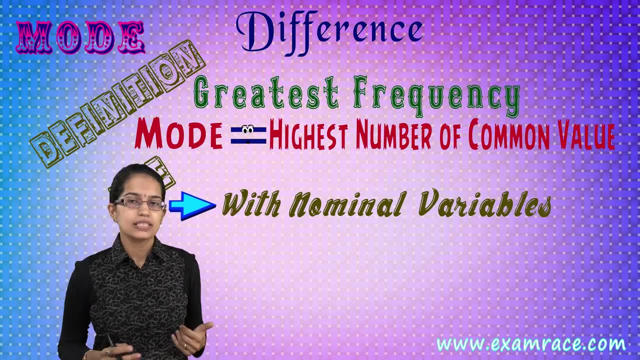 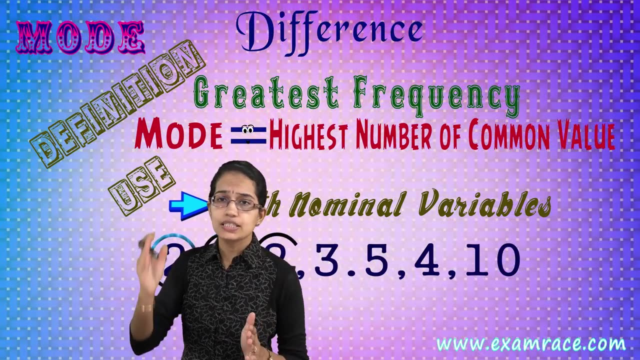 number of instances of a common value that is there is what is mode. Mode is usually seen with nominal values or nominal variables that are there. So when you have just the variables that are there and you find out which instance has the highest number of cases. 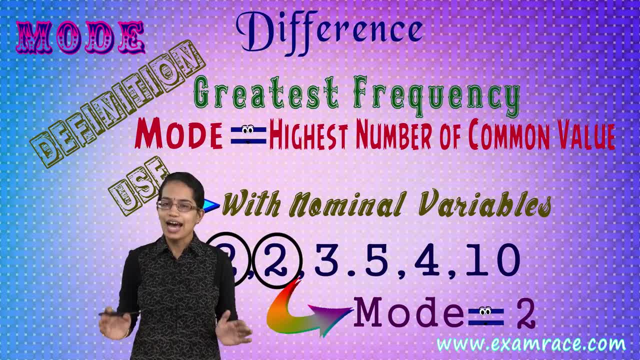 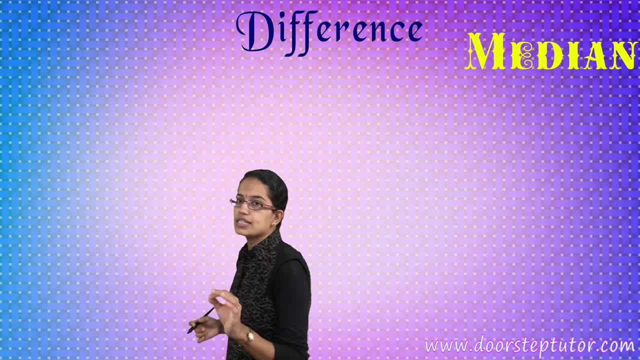 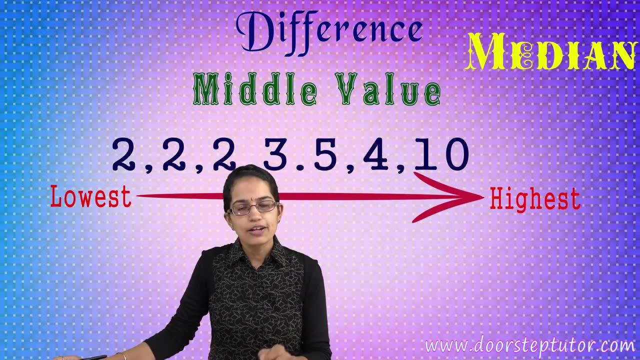 it is just the frequency you are trying to focus on, and that is mode. The last one is a median. What is median? Median, as we said, is the middle value of the distribution. So you arrange the scores from lowest to highest and find out the mid value If it is an odd.